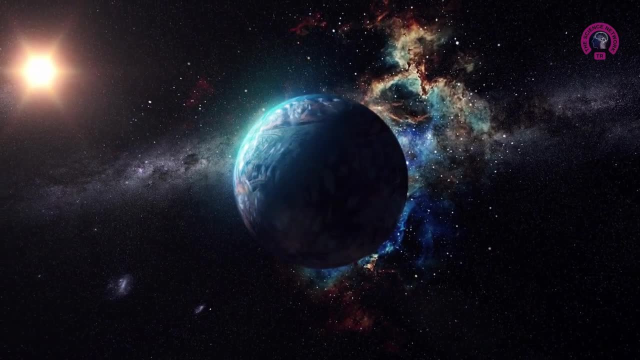 In contrast, the fate of higher-mass stars is the fate of the star itself. The fate of higher-mass stars is the fate of the star itself. The fate of higher-mass stars is the fate of the star itself. The fate of higher-mass stars is far more explosive When their cores have exhausted. 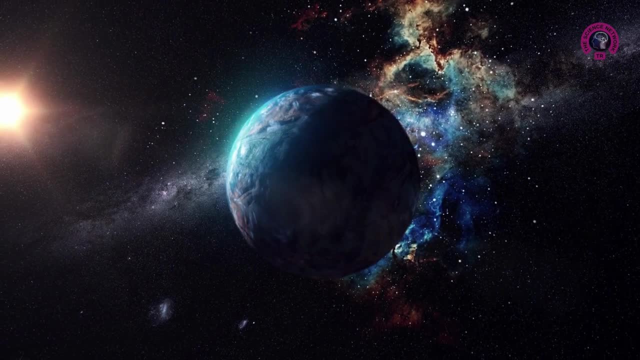 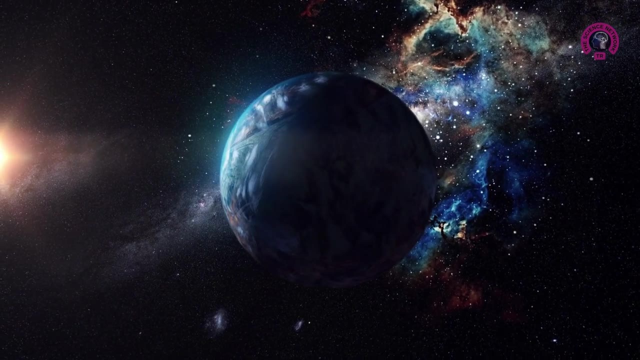 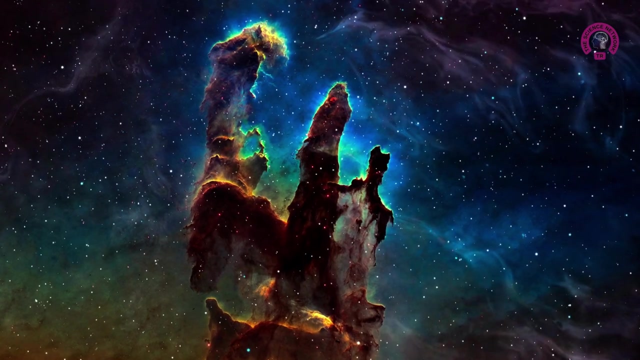 their nuclear fuel. they can no longer withstand gravitational collapse. The result is a cataclysmic event known as a supernova. Supernovae are among the most energetic events in the universe. During a supernova, the star releases an immense amount of energy. 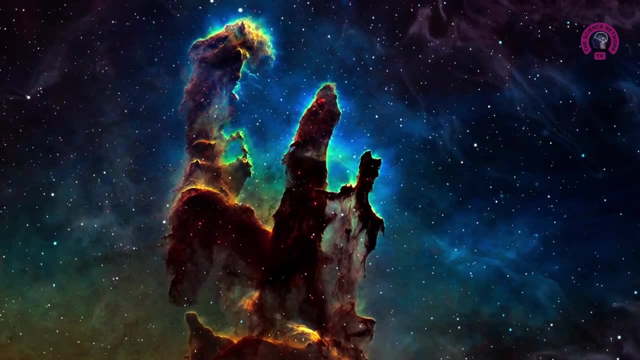 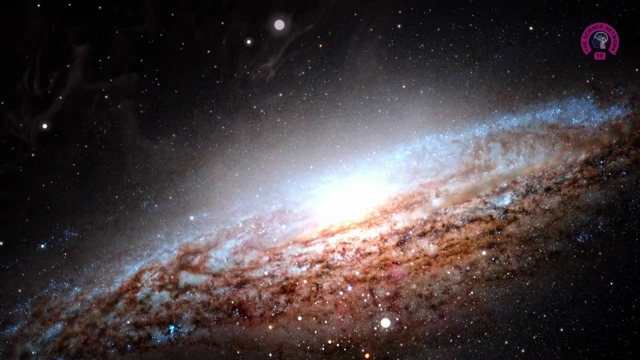 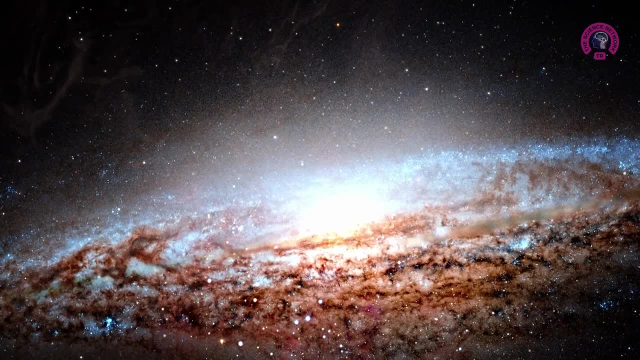 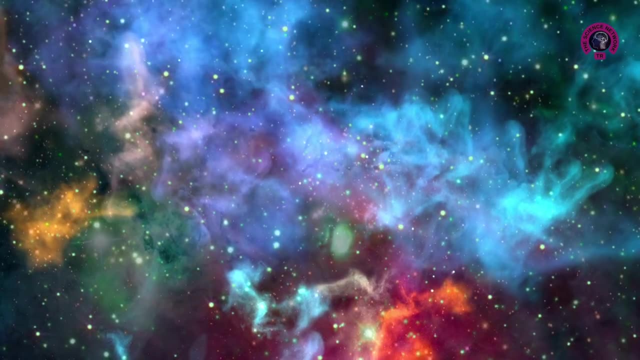 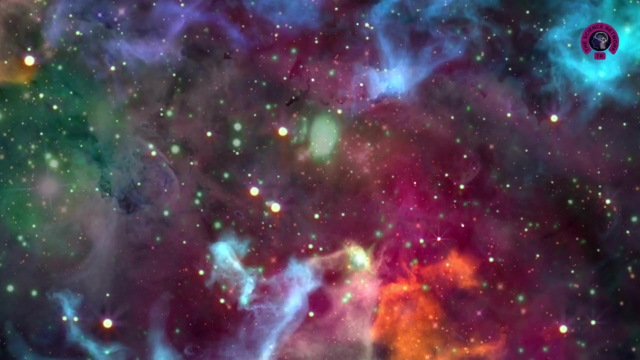 planets and life. The core of a massive star after the supernova explosion may collapse inward, becoming incredibly dense and compact. This remnant is known as a neutron star, which consists mainly of densely packed neutrons. Neutron stars often rotate rapidly and emit beams of radiation which can be observed as pulsars. 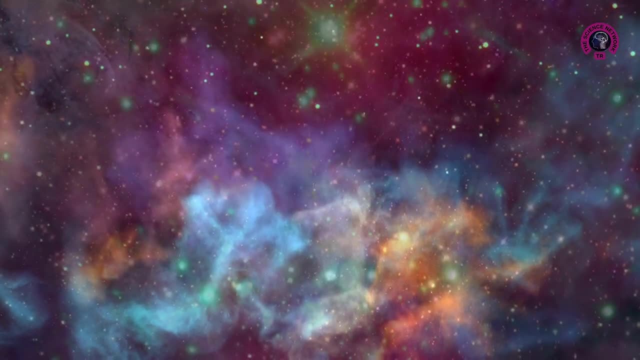 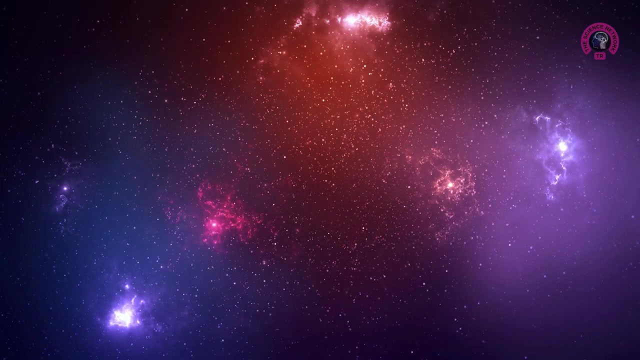 or as a particle of light. In some cases, when the mass of a collapsing star is extremely high, it forms a black hole. A black hole is a region of spacetime with such intense gravity that nothing, not even light, can escape its gravitational pull. The study of stellar life cycles not only reveals 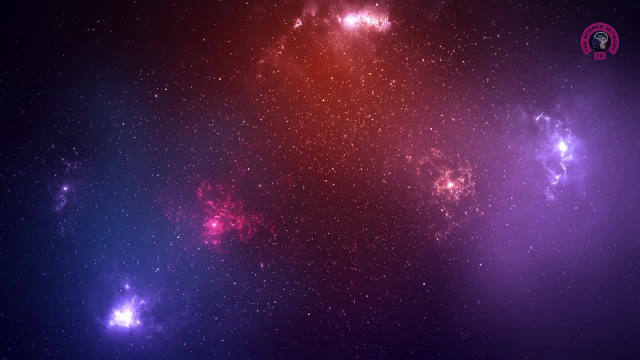 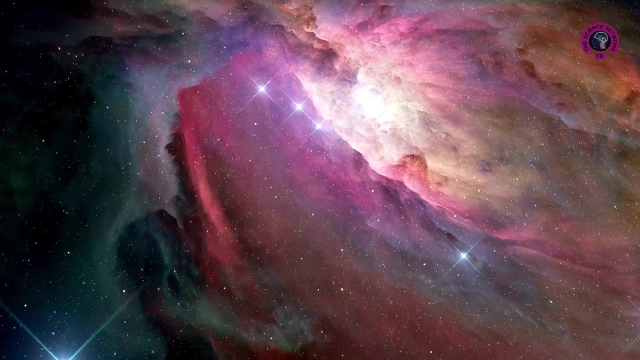 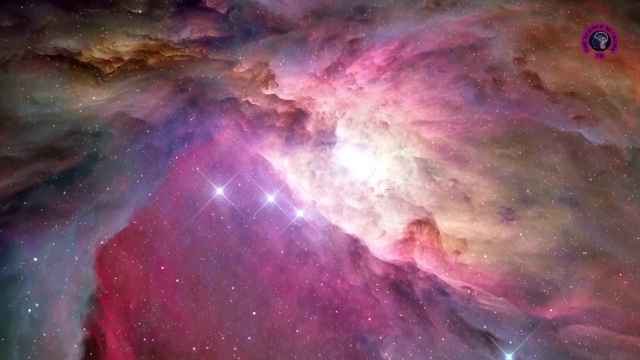 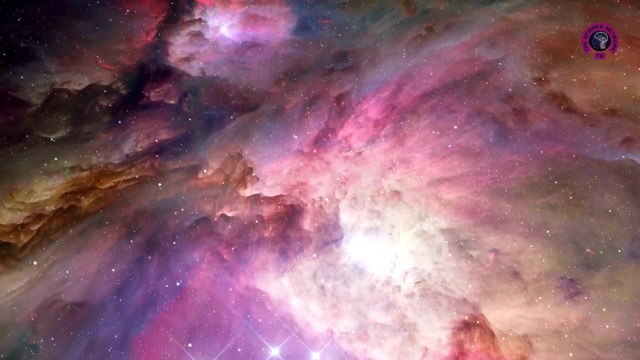 the astonishing transformations stars undergo, but also provides crucial insights into the formation and enrichment of galaxies. By observing and analyzing stars in various stages of their life, astronomers can piece together the intricate history of galaxies, understanding how their composition and structure have evolved over billions of years. In summary, stellar life. 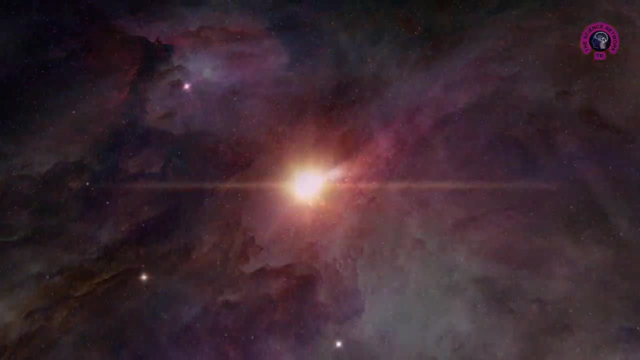 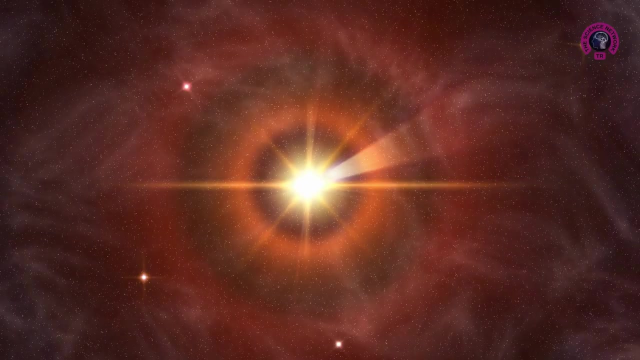 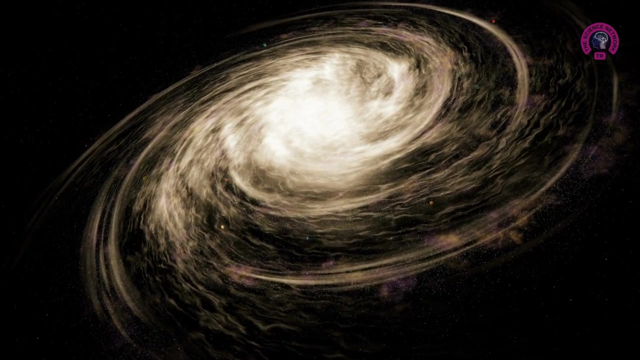 cycles take us on a captivating journey from the main sequence to the explosive finale of supernovae and the formation of fascinating remnants like white dwarfs, neutron stars and black holes. These stages of stellar evolution hold vital clues about the processes that shape our universe. The main sequence represents the stable phase where stars fuse. 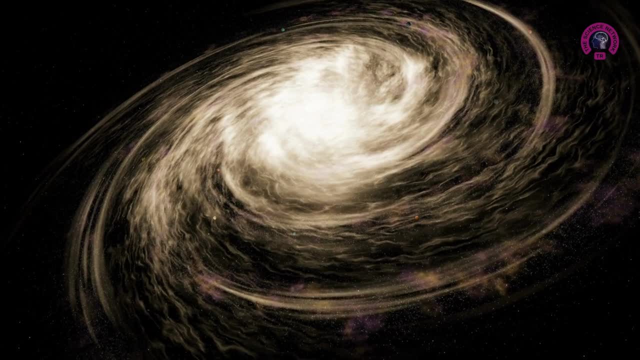 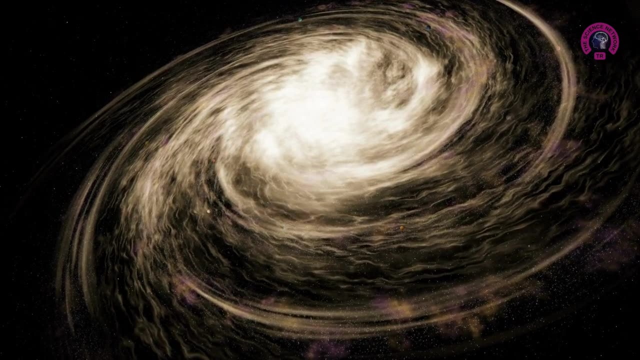 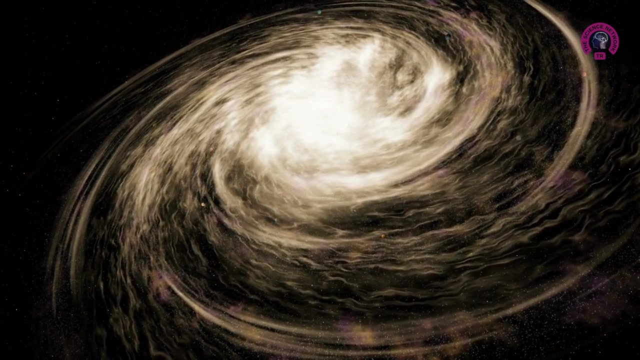 hydrogen into helium, providing the energy that sustains them. Red giants, on the other hand, signify the transition toward the later stages of a star's life, as they undergo significant changes in size, luminosity and temperature. The spectacular explosions of supernovae mark 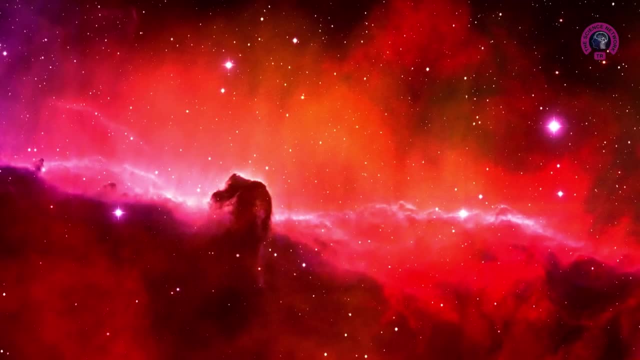 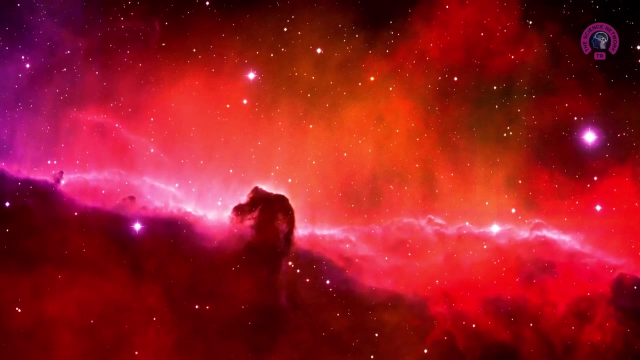 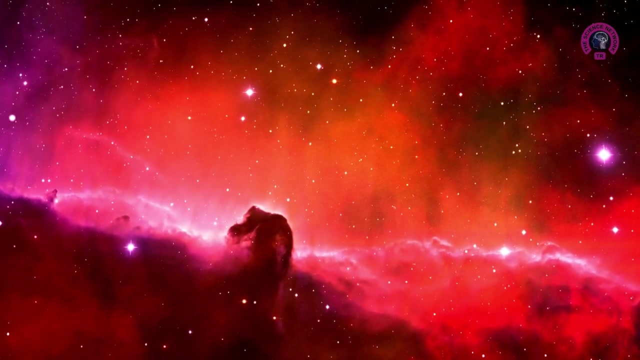 the end of massive stars' journeys, releasing vast amounts of energy and dispersing heavy elements into space. These elements are crucial for the formation of subsequent generations of stars, planets and even life itself. Neutron stars and black holes, the remnants of massive stars, push the boundaries of our understanding of the 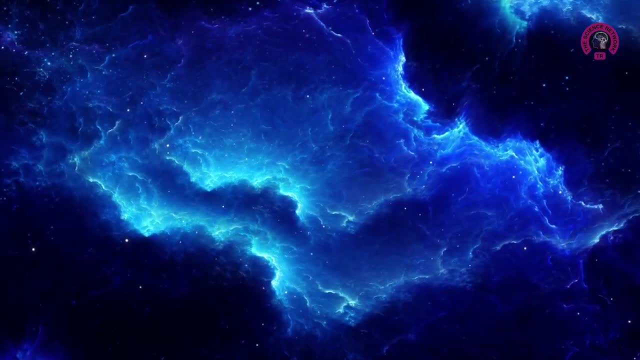 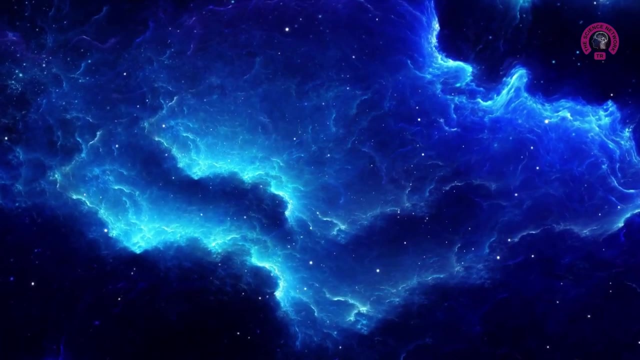 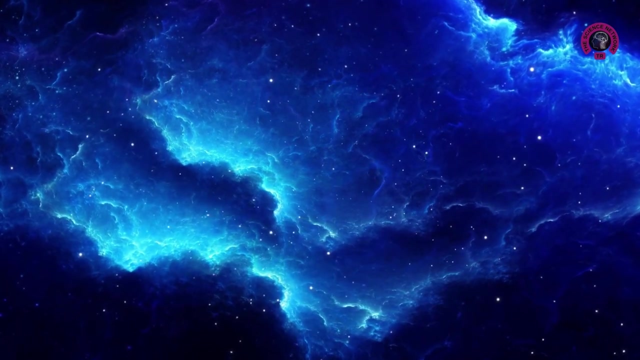 universe. Neutron stars, with their extreme densities and rapid rotation, provide unique laboratories for studying the behavior of matter under extreme conditions. Black holes, with their gravitational pulls so strong that nothing can escape, continue to captivate scientists and challenge our understanding of space and time. 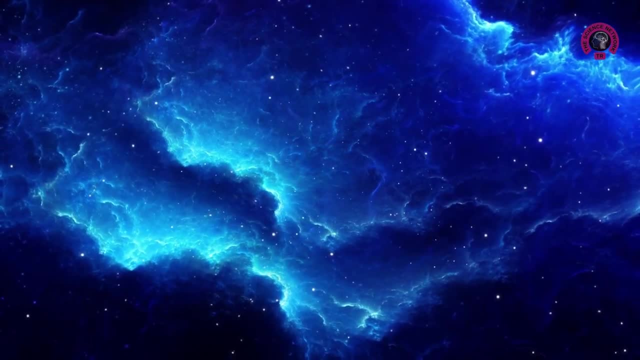 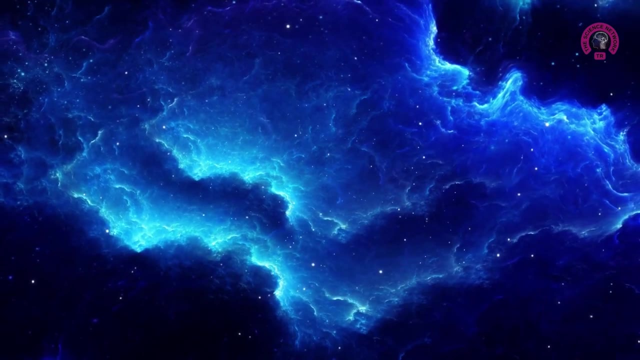 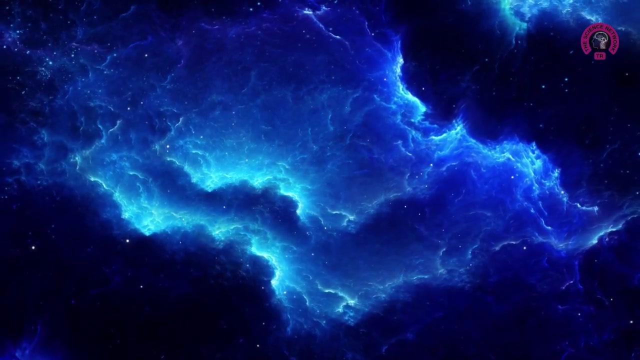 The study of stellar life cycles not only unveils the diverse outcomes of different stellar masses, but also highlights the interconnectedness of celestial objects. Elements forged within stars during their lifetimes are dispersed into the interstellar medium, enriching it and enabling the formation of new stars, planets and, ultimately, life. 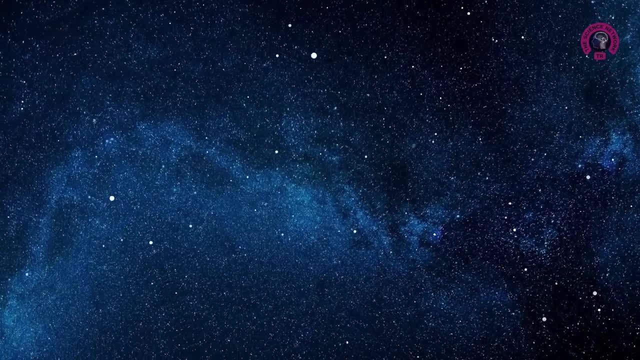 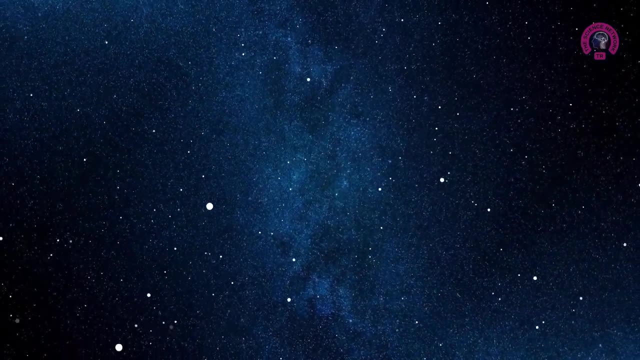 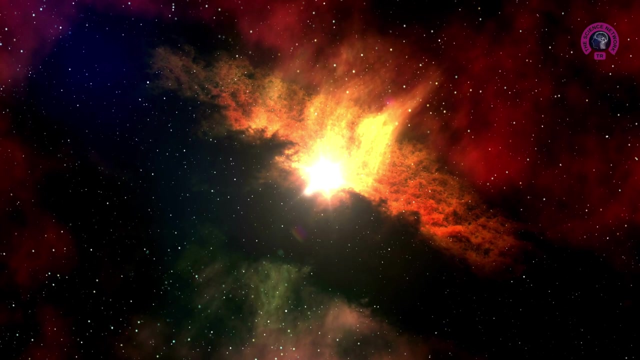 By observing and studying these various stages of stellar evolution, astronomers gain insights into the mechanisms that drive the dynamics of galaxies and the large-scale structure of the universe. Stellar life cycles play a fundamental role in the cosmic cycle of matter and energy, shaping the evolution and composition of galaxies over billions of years. 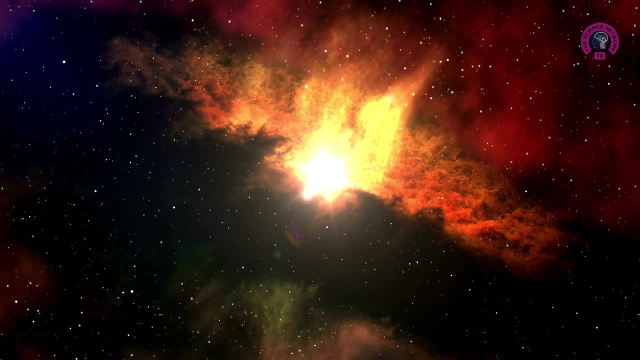 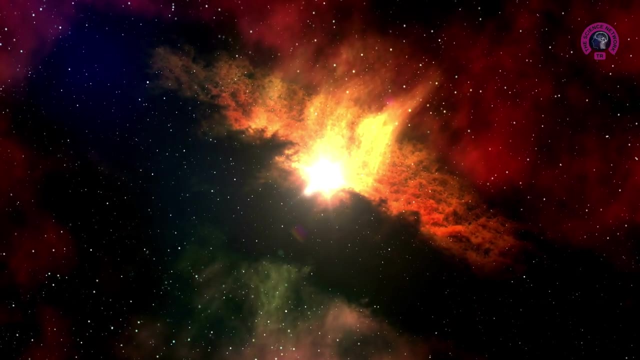 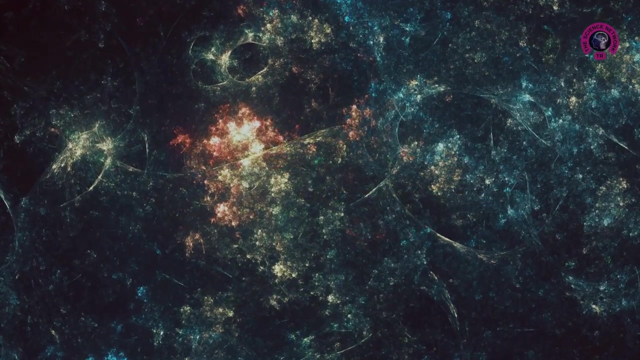 In conclusion, the exploration of stellar life cycles takes us on a remarkable journey from the stable main sequence to the explosive supernova and the enigmatic remnants of neutron stars and black holes. Understanding these stages of stellar evolution not only deepens our appreciation of the universe. 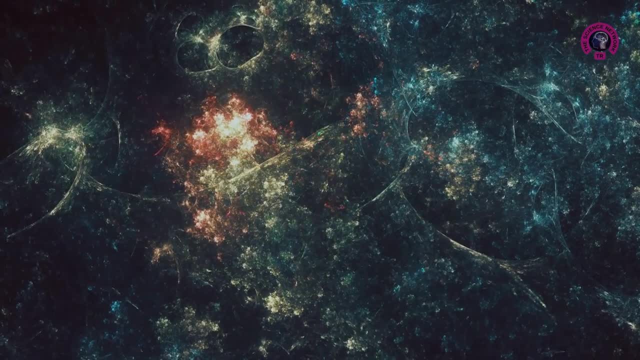 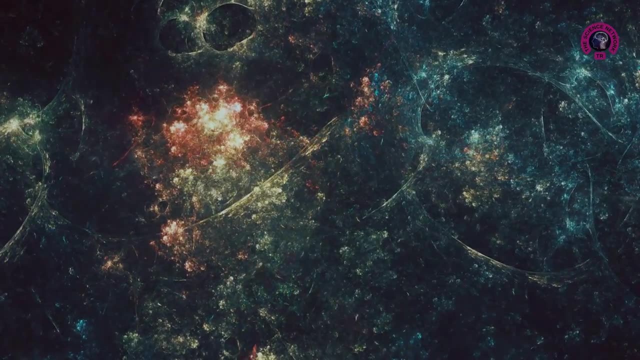 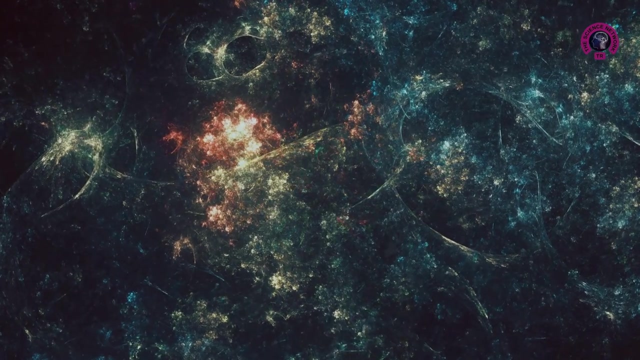 but also provides invaluable knowledge about the origins and evolution of galaxies and the intricate interplay between stars, matter and the cosmos. In our next episode, we will delve into the fascinating realm of stellar structure, properties and variability. Thank you for watching.